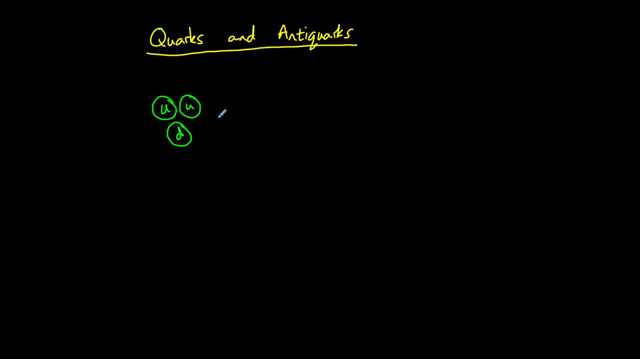 Quarks are fundamental particles that cannot exist on their own. They must be combined with other quarks or antiquarks to form hadrons. There are six types of quarks: Up down, top, bottom, charm and strange. We will only focus on up down and strange quarks. 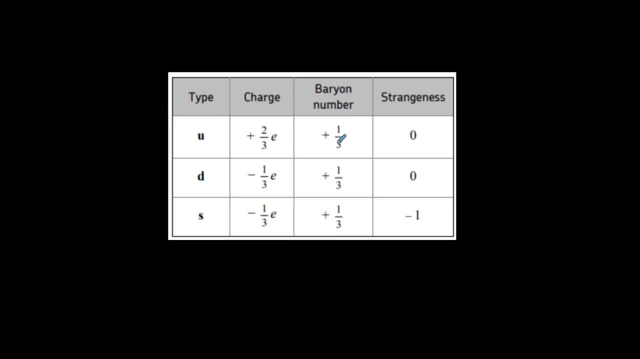 All quarks have a barrier number of plus one. The up quark has got a charge of plus two thirds the elementary charge, While the down and strange quarks have a charge of minus one third. Only the strange quark has got strangeness. 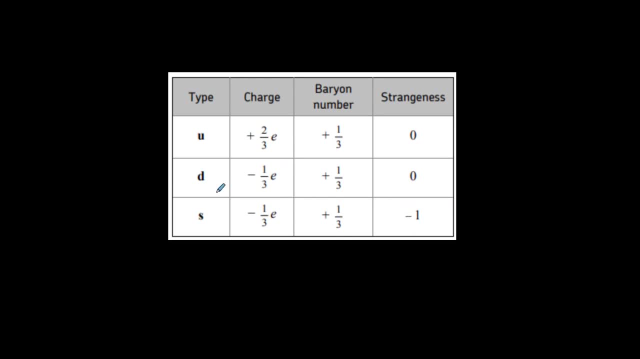 A strangeness of minus one. strangely, For every type of quark there is an antiquark with the opposite properties. For example, an anti-strange quark has a charge of plus two thirds e A barrier number of minus one. A barrier number of minus one third. 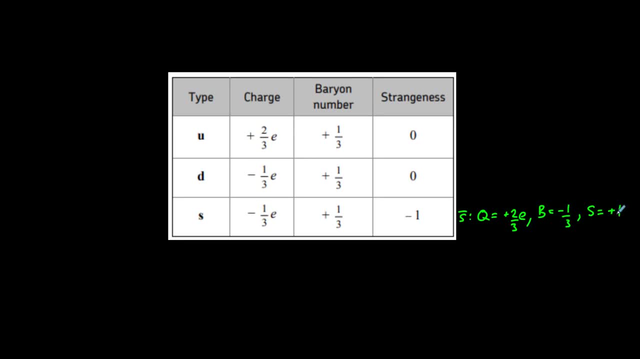 And- a strangeness- of plus one. All baryons are made of three quarks. For example, a proton is made of two up quarks and one down quark. U U D. From this we can deduce its properties: An up quark has a charge of plus two thirds. 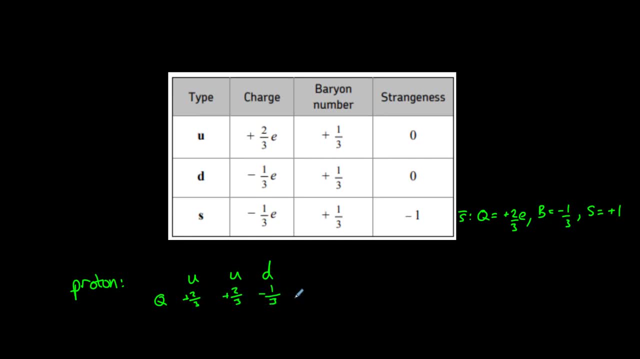 And a down quark has a charge of negative one third, Giving us a total charge of plus one, As we would expect with a proton. They each have a barrier number of one third, Giving us a barrier number of one Again, as we would expect for a baryon such as a proton. 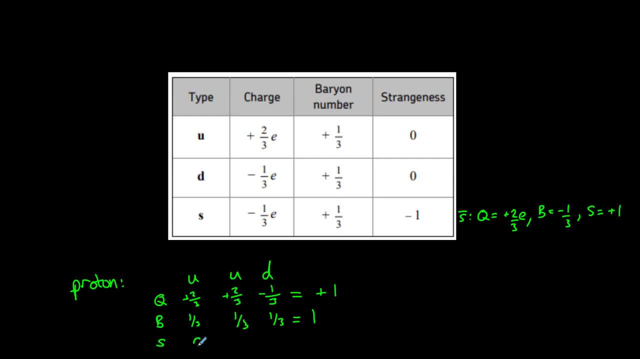 We also know that a proton has no strangeness, And that is true because the up and the down quarks each have zero strangeness too. Similarly, a neutron is made of two down quarks and one up quark, Giving it a total charge of zero and a barrier number of one. 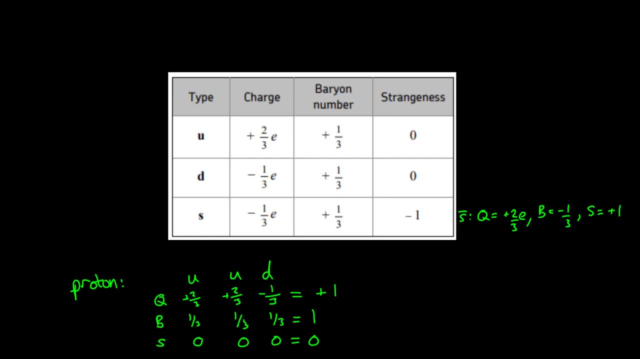 An antibaryon, such as an antiproton or an antineutron, are made of antiquarks. So, for example, an antiproton is made of two up quarks and one down quark, Giving it a total charge of minus one and a barrier number of minus one. 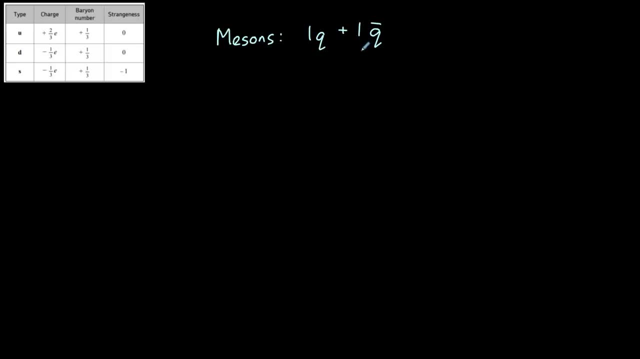 Mesons are each made of one quark and one antiquark. This means that they have a barrier number of zero. As the barrier number of the quark is zero, It is cancelled out by the barrier number of the antiquark. The up down and strange quarks and their respective antiquarks can produce nine different combinations of mesons. 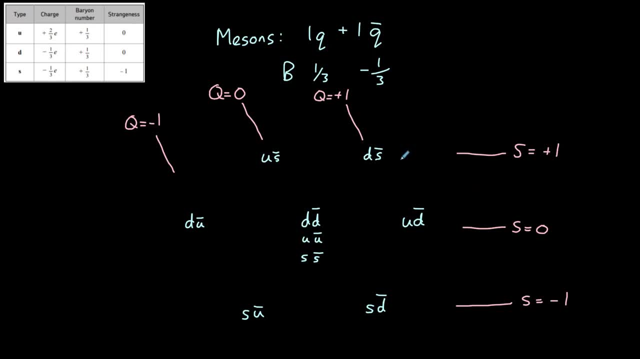 Those that are only made of up down, anti-up or anti-down quarks we call pions, And they have a strangeness of zero because they don't have any strange quarks. Those that contain strange or anti-strange quarks. 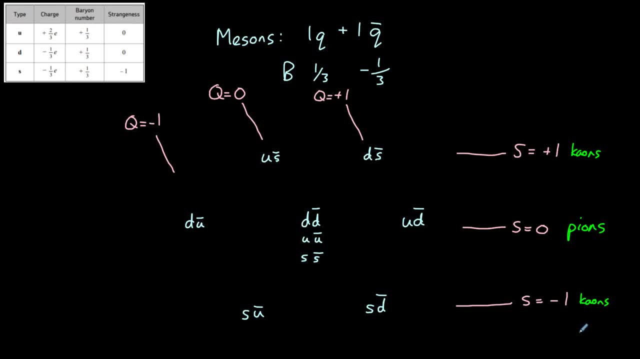 We call chions, And these particles will have a strangeness. Each pion and chion can be expressed as plus, minus or zero, based on their charge. Although there are nine combinations, Note that three of them the down- anti-down, the up- anti-up and the strange anti-strange. 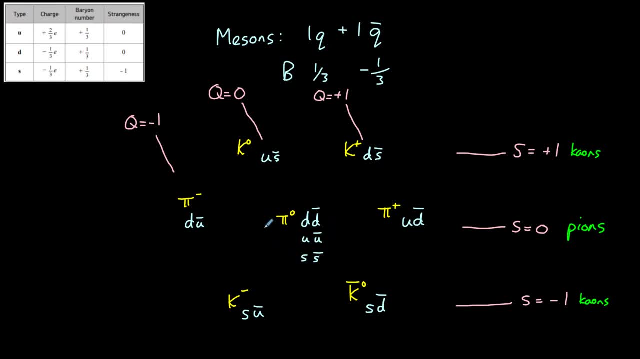 All have a charge of zero and a strangeness of zero, So we call them pi zero particles. This diagram is a convenient way of representing The possible Pions and chions that are formed using up down or strange quarks and antiquarks. 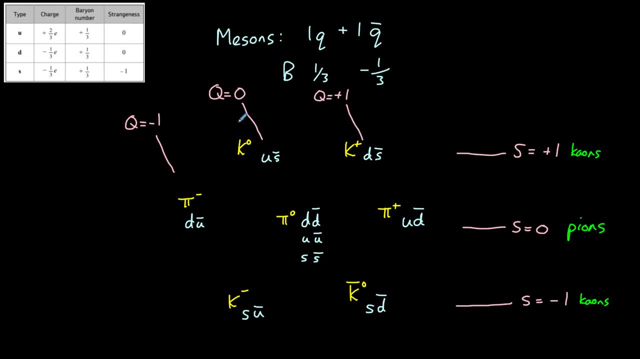 You can see that in these lines They have the same charge. These are negative, These are neutral, These are positive, And in these horizontal lines they have the same strangeness: Plus one Zero for the pions And negative one. 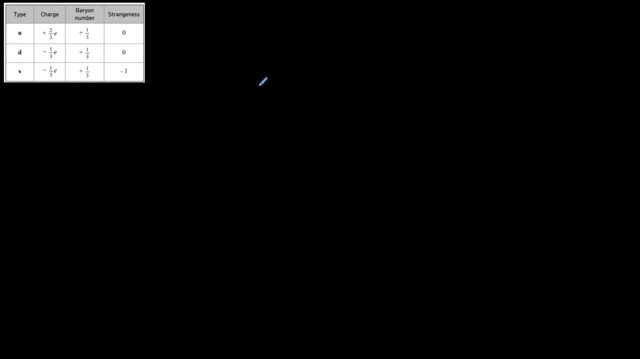 If we know the properties, the charge and the strangeness of a meson, We can easily deduce its quark composition. For example, A pi minus particle must have a strangeness of zero because it's a pion And a charge of minus one. 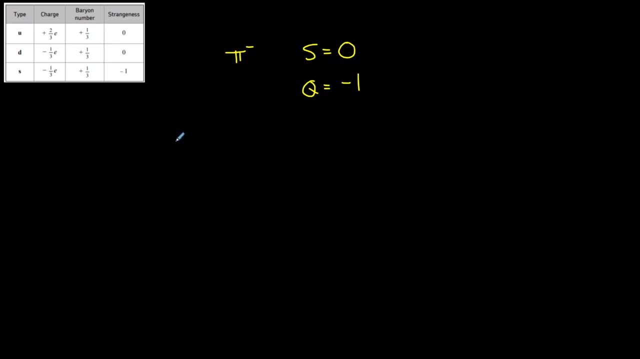 The only quark-antiquark combination that can produce these properties Is a down quark And an anti-up quark, Similarly a k plus quark. A positively charged chion Must have a charge of positive one And a non-zero strangeness.